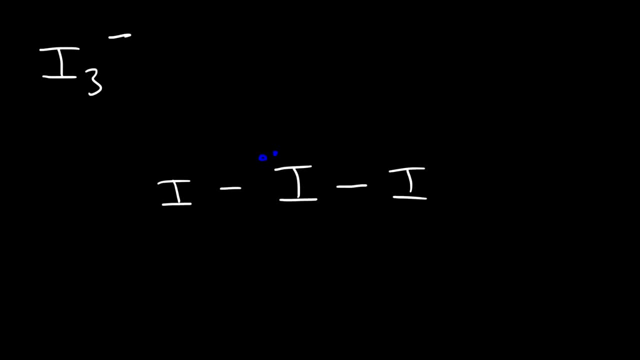 The whole thing is an ion. Now the middle one has three lone pairs And the other two also has three, But the geometry it's straight, It's a linear molecular geometry. Now, the next type of molecular geometry that you need to know is the trigonal. 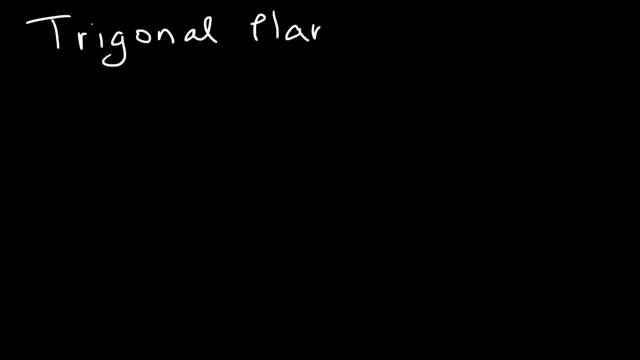 Planar structure. When you hear the word tri, what do you think of? Tri represents tree And planar means it's flat as a paper. A good example of this structure is BH3.. So you have boron at the center. 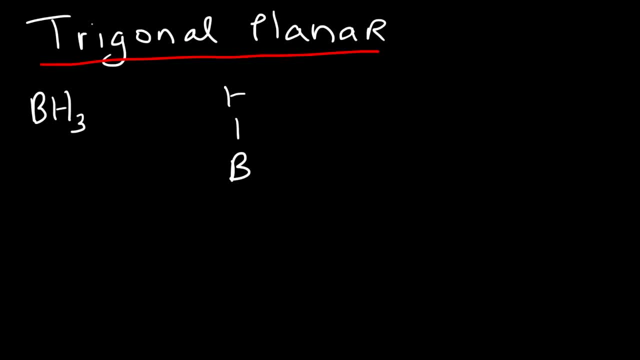 And the three hydrogen atoms are going to be spaced as far apart as possible. So it looks like this: Now, a full circle represents an atom. It has an angle of 360 degrees And if you divide that by three you can get the bond angle between hydrogen atoms. 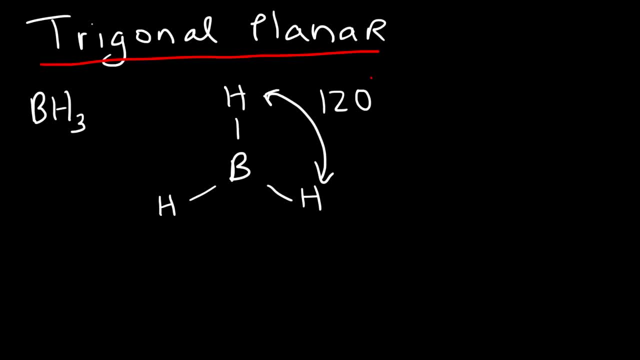 And so the bond angle for a trigonal planar structure is 120, which is 360 divided by three. Some other examples of a trigonal planar structure is COCl2.. So in this structure carbon has a double bond to an oxygen. 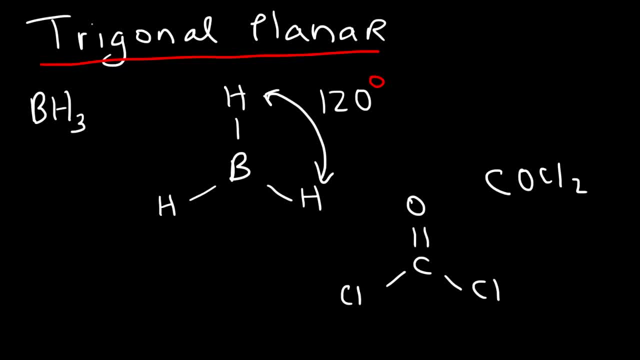 And it's attached to two chlorine atoms. So anytime you have an atom at the center surrounded by three things, And if the central atom doesn't have any lone pairs, then what you have is a trigonal planar structure With a bond angle of approximately 120.. 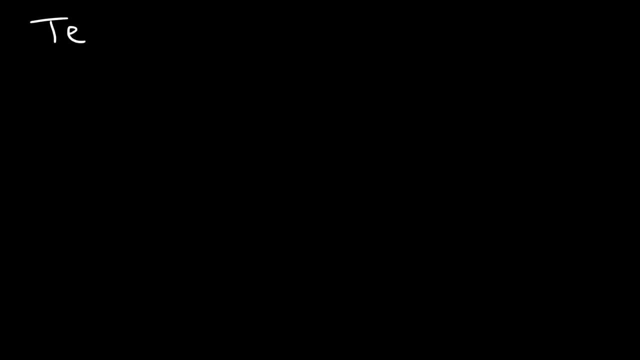 Now the next structure that we need to talk about is the tetrahedral molecular structure. So when you hear the prefix tetra, what do you think of? Tetra is equivalent to four. So therefore, in this structure, we're going to have an atom surrounded by four other atoms. 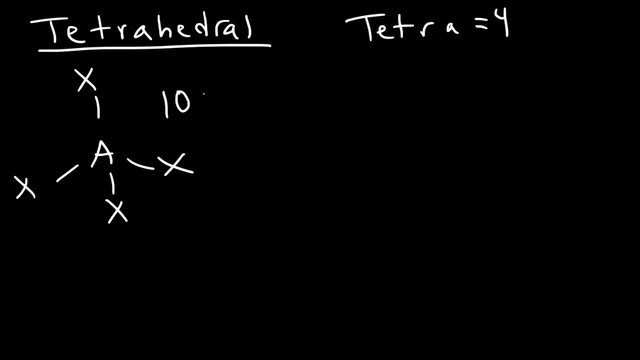 And that's the tetrahedral structure with a bond angle of about 109.5.. So methane fits this example. So in methane we have carbon in the middle, surrounded by four Hydrogen atoms. Now, this is not a two-dimensional structure. 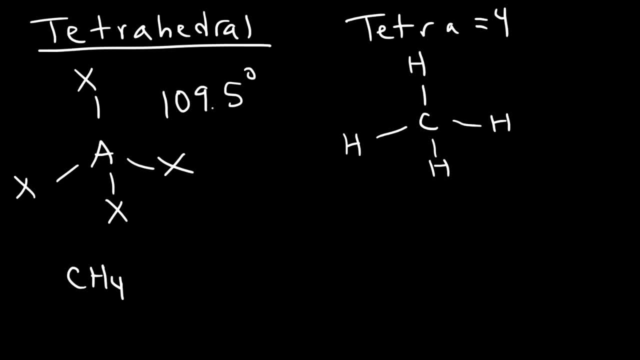 It's a three-dimensional structure Because if you take 360 divided by four, you get 90.. And it's not 90,, it's actually 109.5.. Based on the way these atoms arrange themselves in three-dimensional space. Another example of a tetrahedral structure is silicon tetrafluoride. 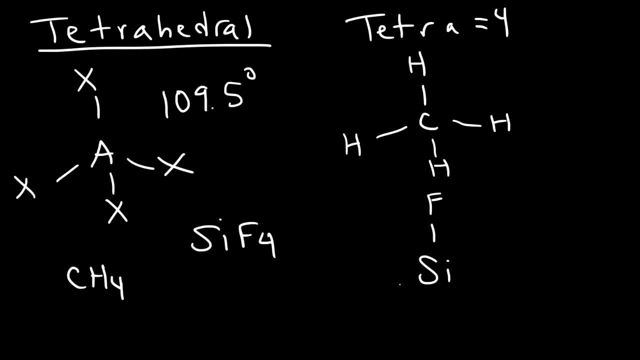 Like carbon, silicon is surrounded by silicon tetrafluoride. It's surrounded by four atoms, In this case four fluorine atoms instead of four hydrogen atoms, But the structure, the geometry, is very similar. You just have different atoms. 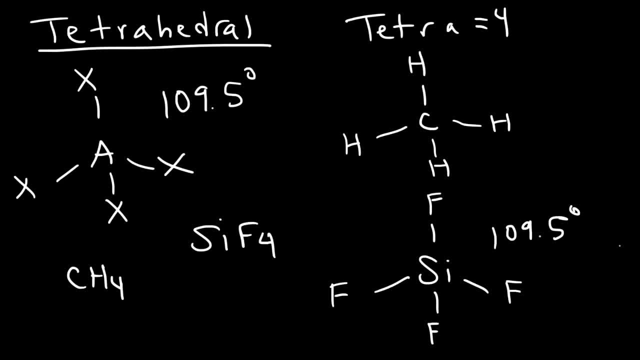 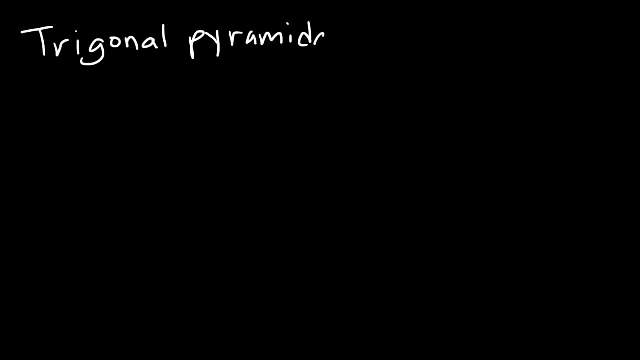 The bond angle is still approximately 109.5.. Now the next structure that you need to know, if you have a test coming up, is the trigonal pyramidal structure. Once again we hear the prefix tri, So there has to be three of something. 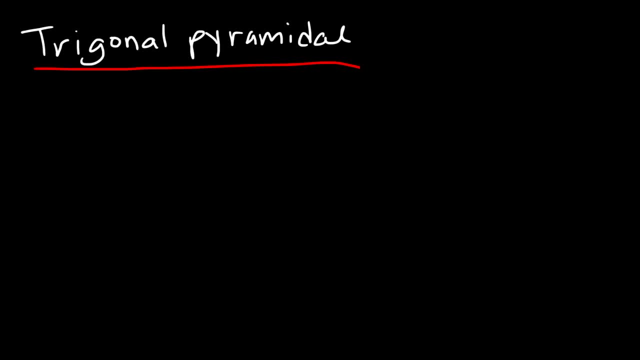 Now this is different from the trigonal planar structure. The trigonal pyramidal structure has an atom at the center with a lone pair. Now that atom is still surrounded by three other atoms, So it looks like this. That's the trigonal pyramidal structure. 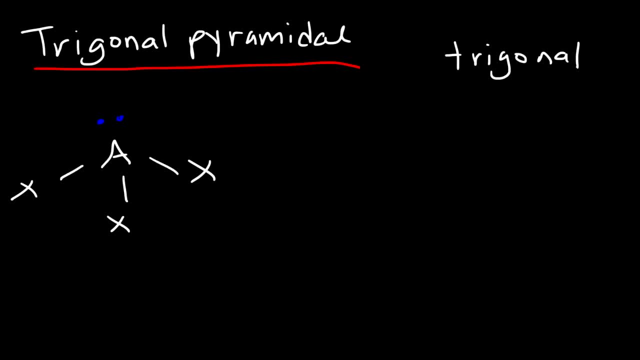 Now just to compare it with the trigonal planar structure. I'm just going to draw this right next to it so you can see the difference. The trigonal planar structure doesn't have any lone pairs on the central atom, It's simply surrounded by three other atoms. 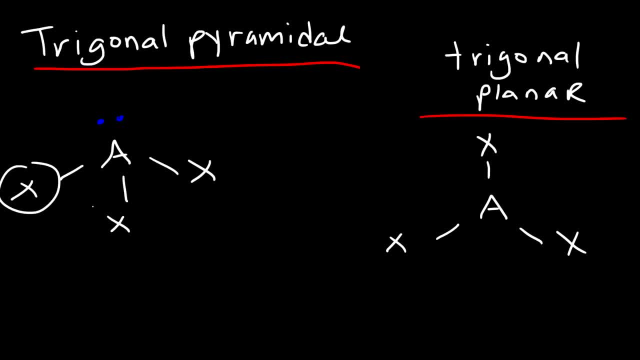 The trigonal pyramidal structure has three atoms attached to the central atom plus a lone pair, So it has four things. A good example of the trigonal pyramidal structure is NH3, ammonia. In this structure, nitrogen has one lone pair. 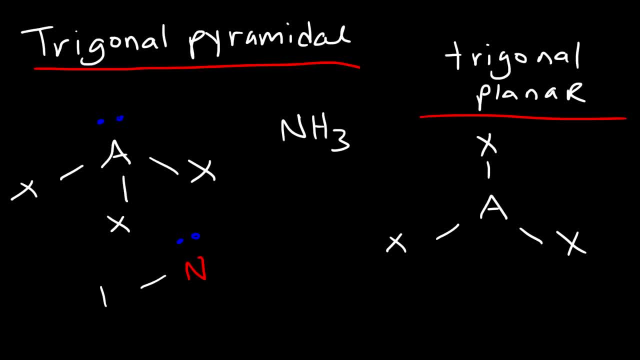 and it's attached to three hydrogen atoms. Another example is pH3.. So, if you notice something, I just want to point something out: LH3.. Elements that have the trigonal planar structure tend to be in group 5. Like NH3,, pH3, and ASH3.. 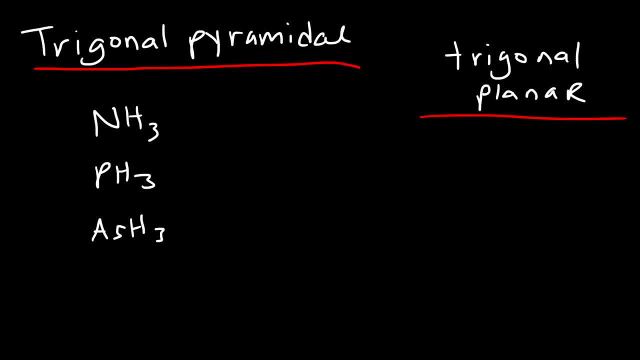 When hydrogen is like the only other atom attached to it, And the ones that have a trigonal planar structure tend to be in group 3, but not always though. So BH3 is an example. Another example includes ALCl3.. So these elements are in group 3a. 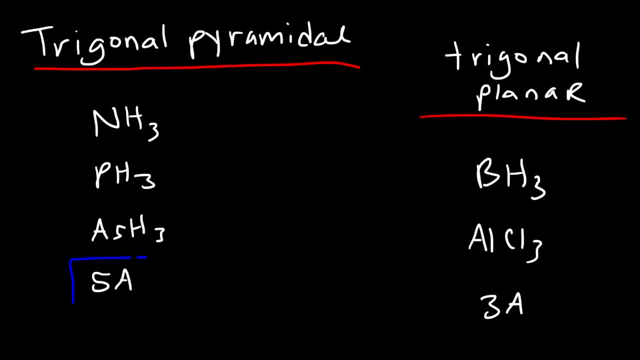 and these elements tend to be in group 5a. So that's another quick way to identify which one is going to be trigonal planar, which one is going to be trigonal pyramidal, If there's no double bonds involved. 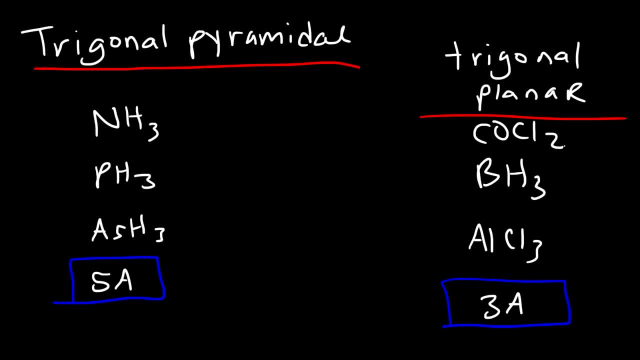 Because we did have the example where it was like COCl2, but the carbon attached to an oxygen had a double bond. If there are no double bonds, for the most part these elements will be in group 3a and these will be in group 5a. 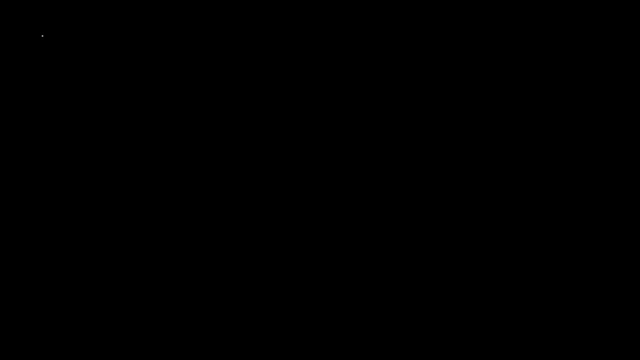 So that's the pattern I've seen. Now, going back to the trigonal pyramidal structure. there's one other thing I need to mention, And that is the bond angle. I'm going to use ammonia as an example. So the bond angle for ammonia. 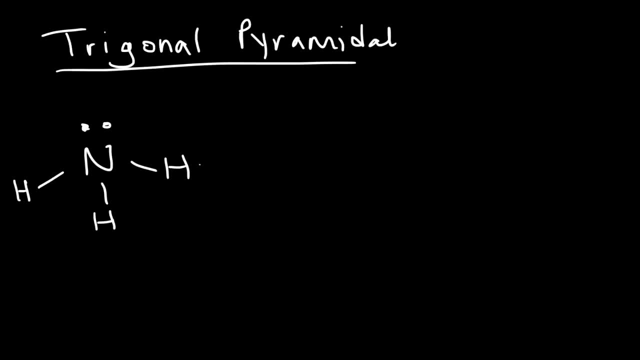 make sure you know this, because it's a common test question. It's about 107 degrees, And so that's it for this example, The trigonal pyramidal structure. Just wanted to mention that before I forgot it. Now, the next geometry you need to be familiar with: 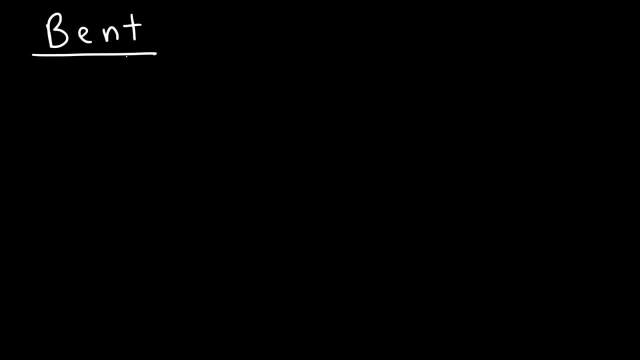 is a bent molecular geometry, And a good example for this one is water. Water has a bent shape. Oxygen contains two lone pairs, And those two lone pairs causes the hydrogens to be in a bent structure. Now perhaps you've seen water drawn like this. 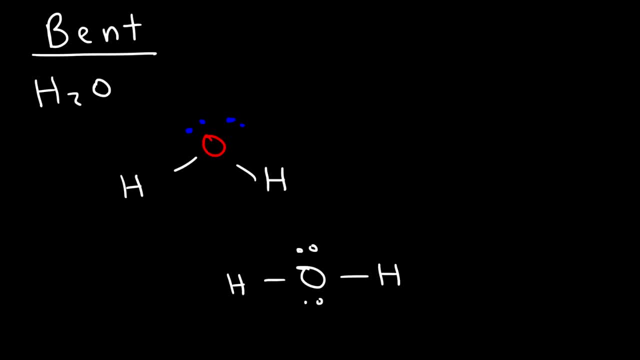 And this is a common mistake, so you don't want to do it- But rather the lone pairs, causes the hydrogens to be bent with respect to each other And the bond angle for water is 104.5 degrees. Another example of a bent structure. 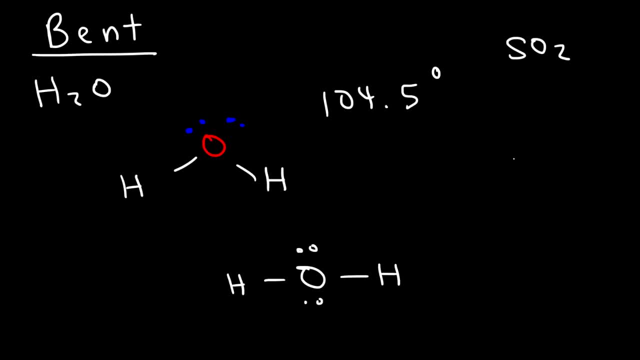 is the sulfur dioxide molecule. In this structure, sulfur has two oxygen atoms. One has a double bond and the other has a single bond, And sulfur also has a lone pair. It doesn't have two lone pairs in the case of oxygen, But it has one lone pair. 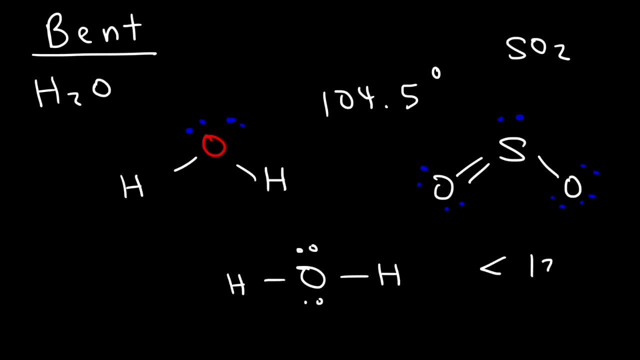 And the bond angle is less than 120.. Notice that this is similar to a trigonal planar structure In the sense that it has two atoms and a lone pair. A trigonal planar structure has three lone pairs with a bond angle of about 120. 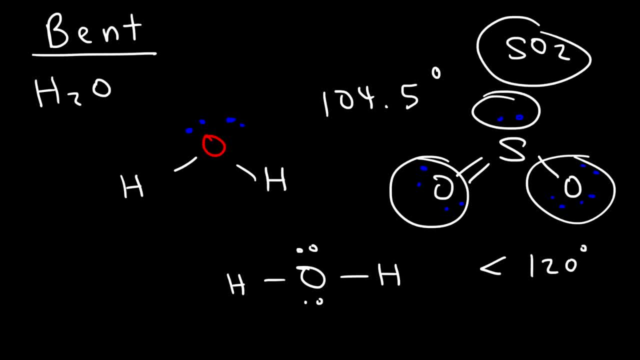 So SO2 has three things: Two atoms and a lone pair on the sulfur atom, And that's why the bond angle is similar to a trigonal planar structure. Water is somewhat similar to a tetrahedral structure In the tetrahedral structure. 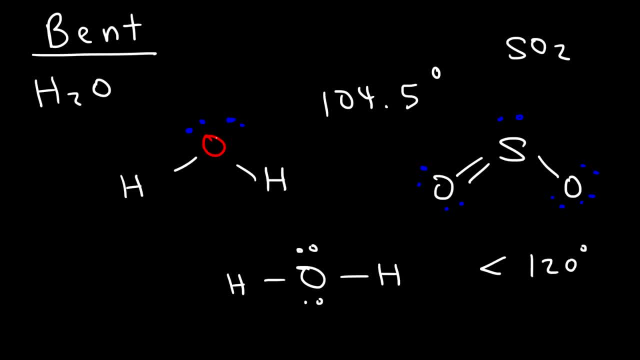 there's four things or four atoms in the central atom. In the case of oxygen, it has four things: two atoms and two lone pairs. That's why the bond angle is close to that of a tetrahedral structure, which is supposed to be 109.5. 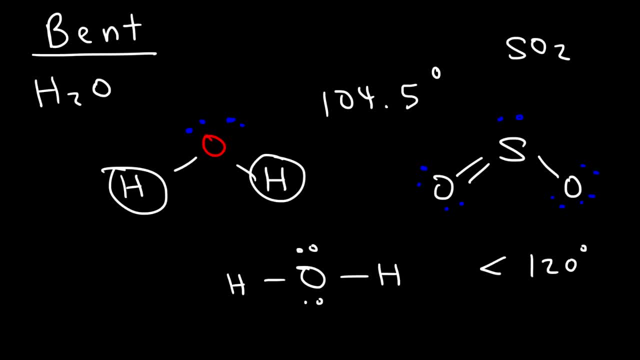 But in the case of water it's actually 104.5.. Now I want to put certain molecules together. So for a tetrahedral structure, in the case of methane it has four groups, It has four atoms attached to it. 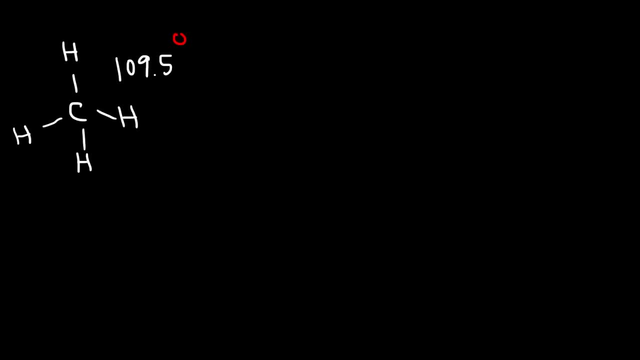 The bond angle is 109.5.. Now if we replace one of those atoms with a lone pair, as in the case of ammonia, we're going to get the trigonal pyramidal structure. And because we still have four things, 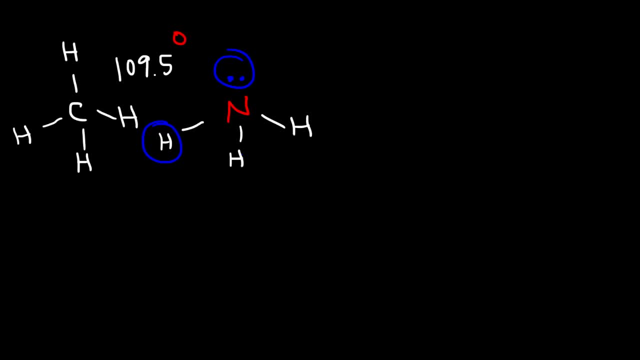 in this case three atoms and a lone pair. the angle is going to be close to 109.5, but it's a little bit less. If you subtract this by 2.5, you're going to get 109.7 degrees. 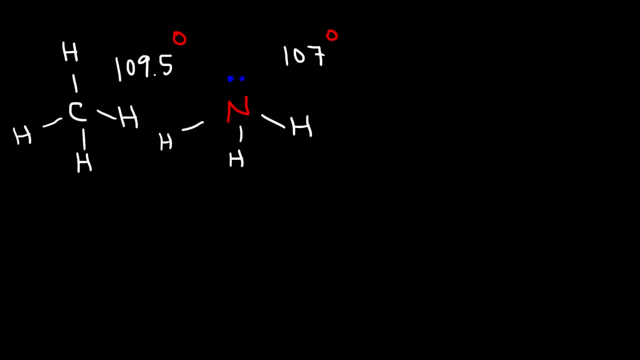 And that's the bond angle of ammonia, with its trigonal pyramidal molecular structure. The next one is water, which looks like this: It has two lone pairs instead of one, But it still has four electron groups: Two, three, four.